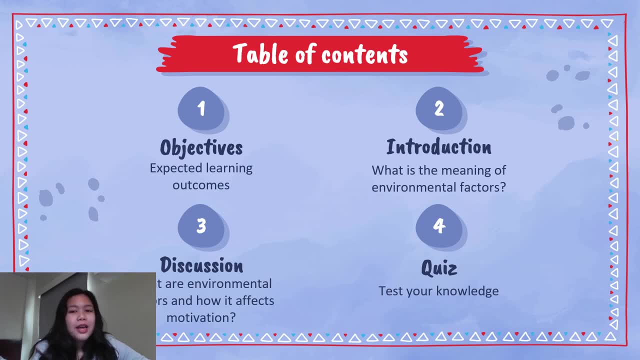 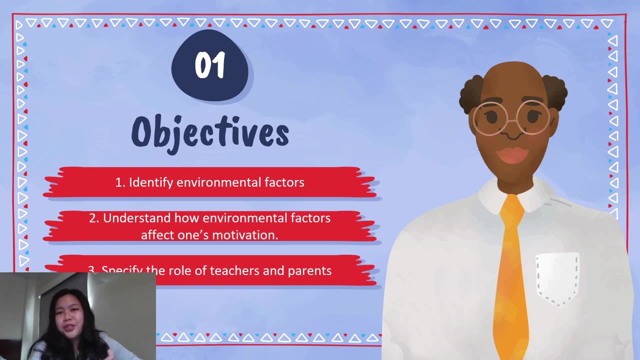 Yes, we're going to have our 10-item quiz And yes, let's begin Objectives. So at the end of this last one, you guys should be able to identify environmental factors. Ano ba, may environmental factors Number two, understand how environmental factors affects one's motivation? 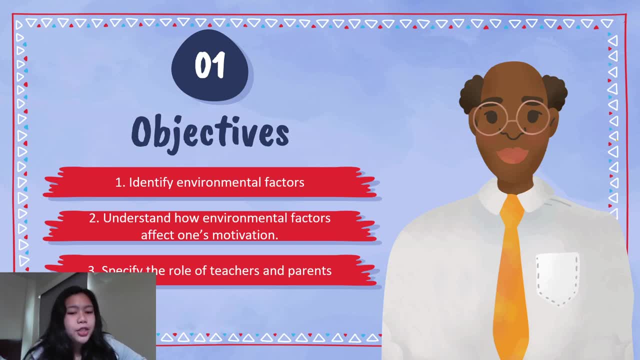 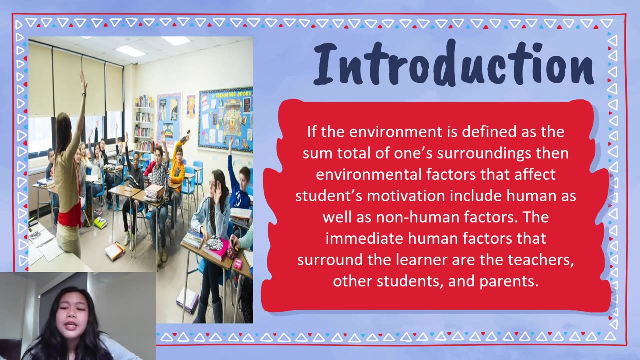 Hmm. Number three specify the role of teachers and parents. So may gagampanan pala yung si teacher at saka si parent. Anyway, without further ado, what is environmental factors? Now, if the environment is defined as the sum total of our surroundings? 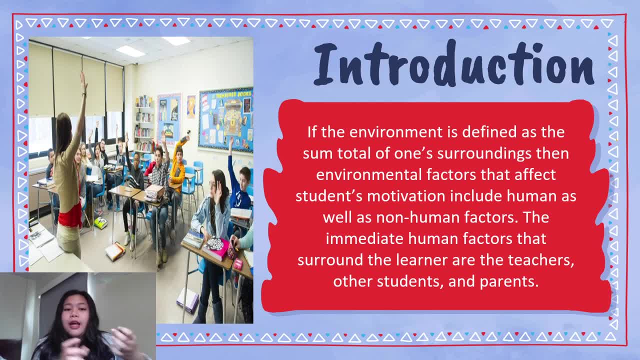 then environmental factors is something that affects student motivations, And that includes two: Human And non-human factors. Now, non-human factors, those are not human, For example, the environment, the surroundings. They are not human, They are just a place. 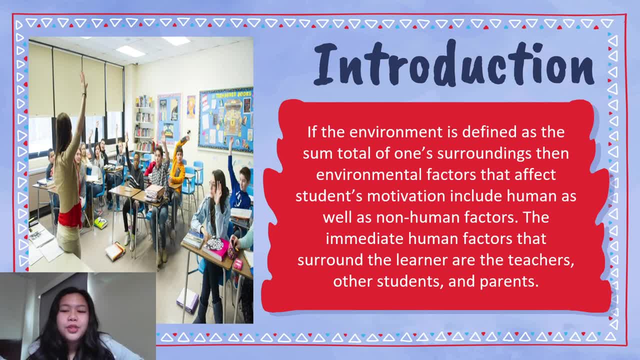 Now, when we say human, those are people that surrounded the learners And that is the teacher, Other students, which are the classmates, And also the parents. The parents are always involved. They are always members of the students. Now we already know what environmental factors are. 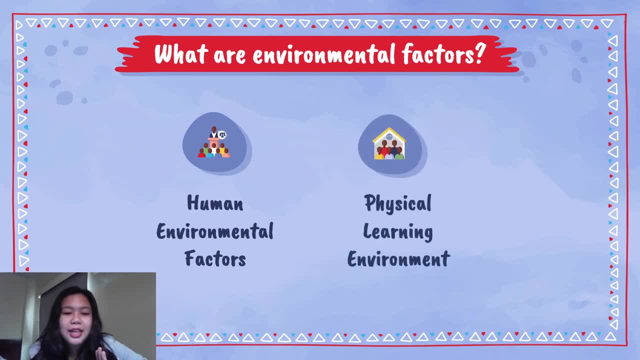 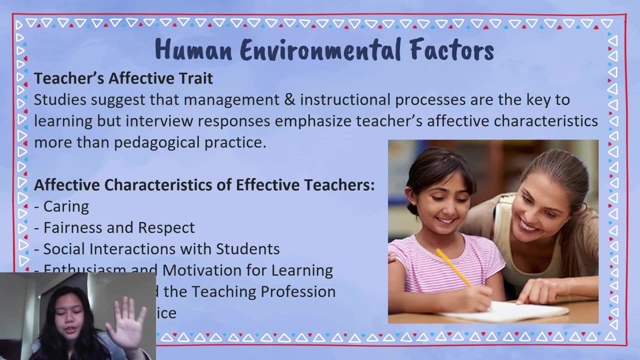 Okay, We have two Human environmental factors and physical learning environment. Again, human environmental factors and physical learning environment. Now, how does that affect? Let's discuss. How does affect, How does human environmental factors affect the motivation? Well, let's begin. 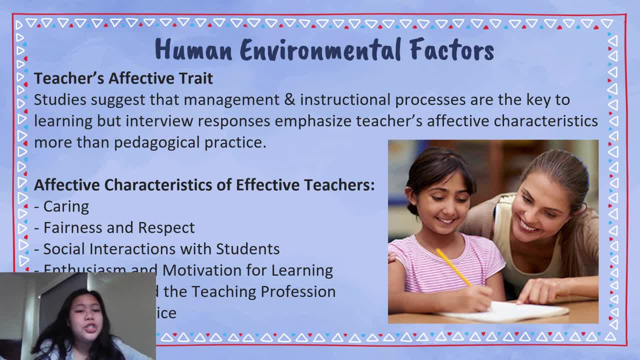 The teachers, teacher itself. Now they say teacher's effective trait suggests that management ng teacher tapos mga instructional process are the key to learning para makaintindi yung estudyante. but now, according to studies, it's the effective characteristics more than pedagogical practices Sa pedagogical 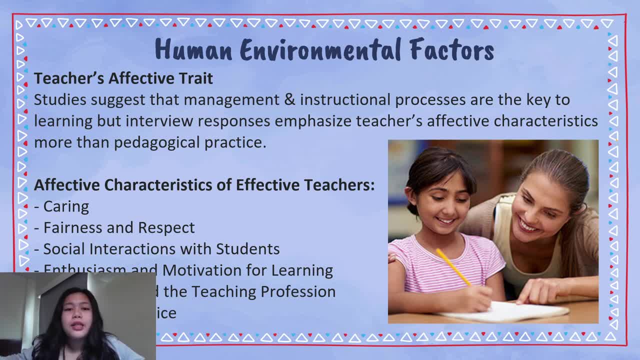 practices. it's the way you manage your students, or how are you going to? maybe you're going to implement rules, punishment, rewards, unable to control them, or you might going to use differentiated instruction able to get the specific or the. what do you call this? the capability, or let them just let the students learn according to their capability? 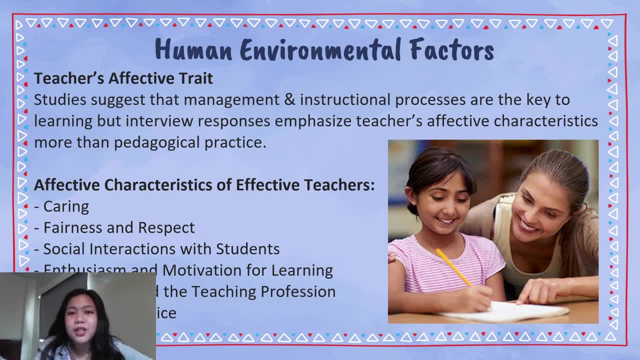 It's not all about those things, it's all about the characteristic of a teacher. now, it's the characteristic of a teacher: what makes the student learn? yes, um, okay, here are the effective characteristic of effective teachers. imagine your, your teacher is caring, caring. si teacher sasabihin mo, ma'am, i'm not feeling well, katulbon ko. 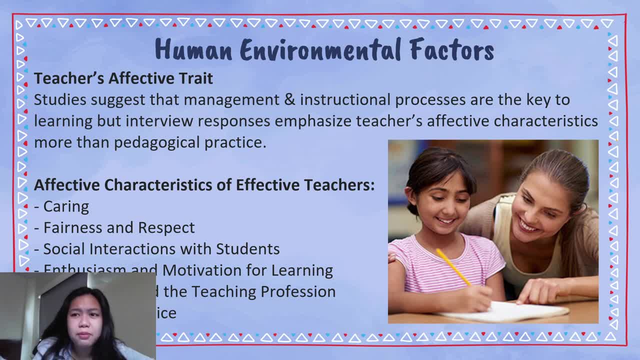 that's a caring teacher. inaantok ka. bakit hindi ka ba natulog? have you slept? uh, did you sleep last night? no, ma'am, okay, you can go to the ano. you can take a nap a little bit and come back to our class. 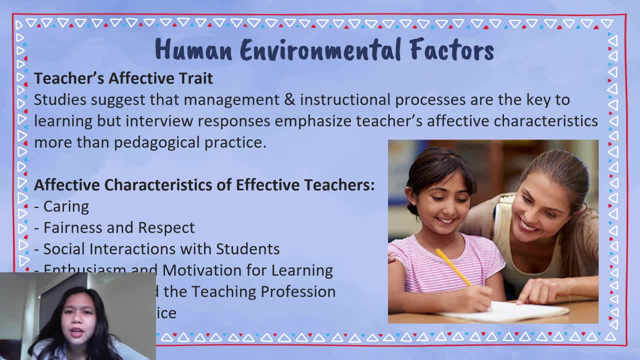 okay, a teacher like that, san kayo makakita ng teacher ng gano' no, next, fairness and respect a teacher who have who, who are fair to his or her students student. no di porket mayaman tong isang student mayaman ang pamilya nito itong papaboran mo. 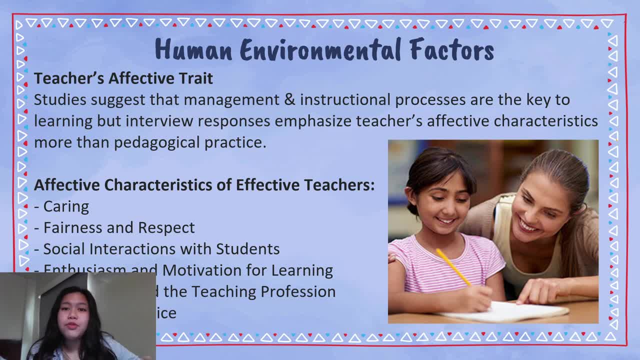 no, you have to be fair with your student, rich or poor? no. and next, social interaction. now, if the teacher, an effective teacher, always have this characteristic, always interact with his or her student. now you know what? um, i'm going to share it to you guys. are you like me, na always hesitant to greet a teacher? hindi mo magawang, good morning, ma'am. 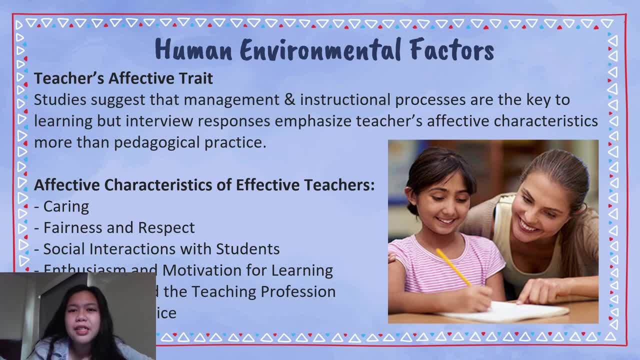 good morning, sir. see, you have this hesitancy, you have this fear to be neglect again, to be disregard again, and that is because it's not our fault. it's not our fault, i think, i think it's one of the teacher's fault. i mean, it's because of that human, environmental factor that that teacher it's herself or his self himself. 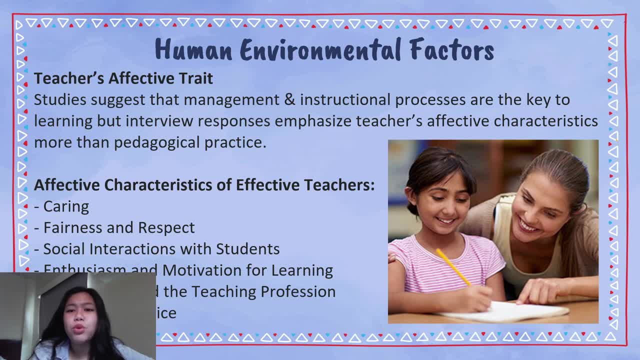 are the factors that we are not motivated enough, because motivated to greet her or to greet him because he himself is not approachable. so, ladies and gentlemen, future educators, you always prioritize interaction. you have to get the heart of a student, even in a simple greeting. greet, pa. 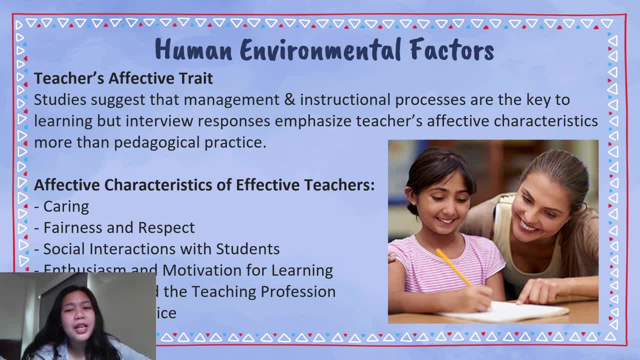 good morning ma'am, oy, good morning inday. oy, good morning dong, because in that way the student, you can light up your student's day. oy, si ma'am pinansin ako ni ma'am friend me ni ma'am ganoon hindi yung. good morning ma'am. 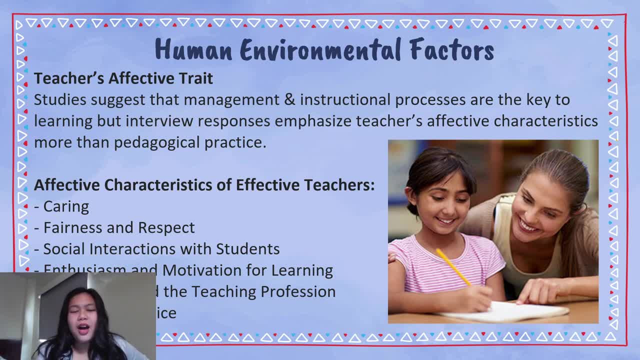 snub lang alam yung may feel ng student. ma-hurt, ma-hurt, yung student like ay may galit pa si ma'am sa akin. ayaw ba ni ma'am sa akin? ma'am, sabihin niya kay sabihin ng sa mama niya, ma hindi na akong magsuschool. parang ayaw ni ma'am sa akin. 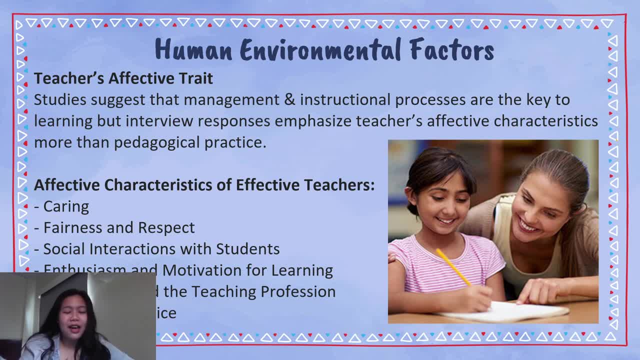 so ganoon ba. so okay again, social interaction has a great impact with your relationship towards your student and, yes, if you interact with them, then there's a high possibility that you can have great quality relationship with your student. ganoon lang yun mga future teachers. 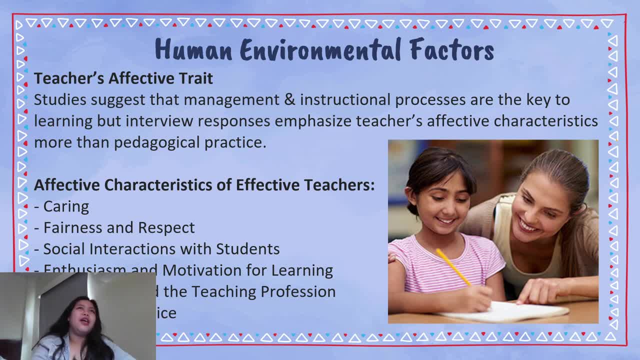 next, enthusiasm and motivation for learning. now, okay, example: you teach filipino or arpan or math. no, most commonly students and um reaction is like: ah, boring na, boring na subject, ayaw akong makinig. eh, matulog na lang ako there, makikipag, usap na lang ako. 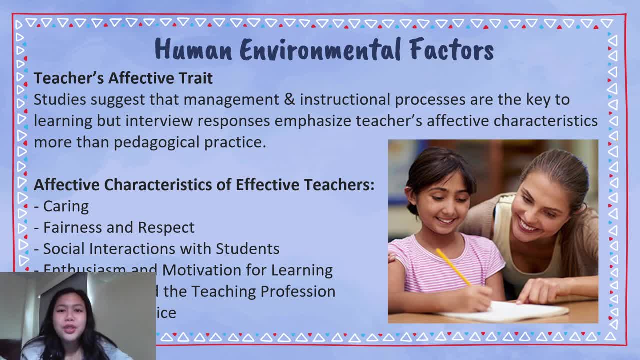 ganoon. now, as a teacher, you should have this enthusiasm to make your student participate. yes, to make your. to make them participate, especially those lower grades. they have this lower, like shorts, attention span towards you. yes, so you have your enthusiasm. your energy should be at the highest peak. 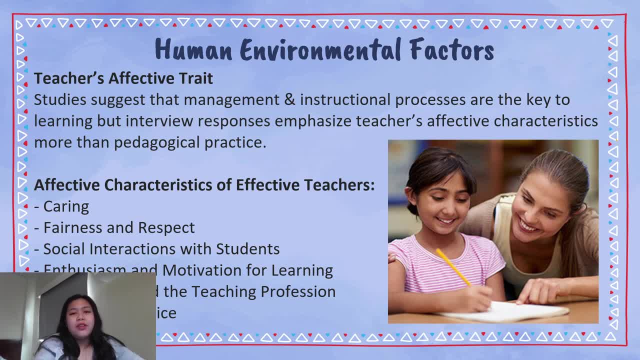 hindi ka dapat mauubusan kasi. how can they get motivated, diba? you should start with yourself as a teacher, motivated to teach, so that they are motivated to learn from you. so, yes, that is one of the characteristic of effective teachers. moreover, we also have attitude. 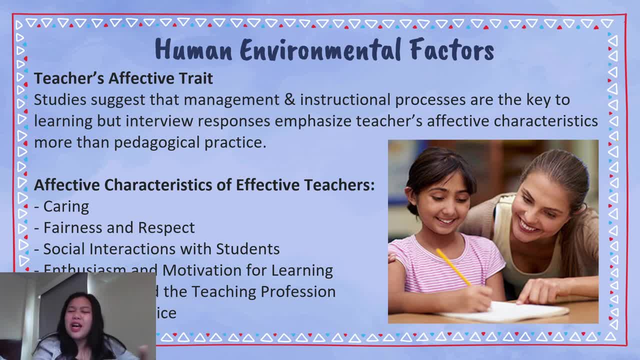 toward the teaching profession. so parang connectado din. no, your attitude toward teaching. are you that kind of teacher na basta makasweldo ng fights na? or are you that kind of teacher who are more focused on the modeling, modeling of students mind. are you that kind of? 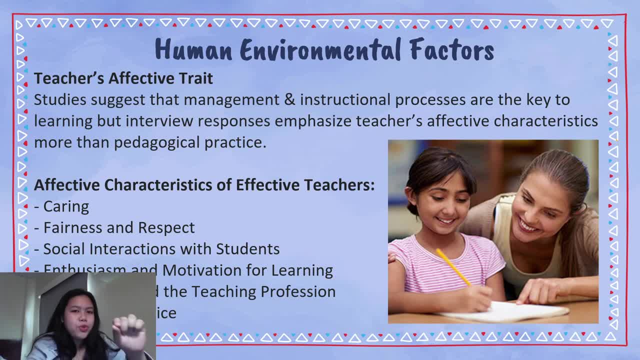 teacher na um magsulat kayo dyan page 1 to page 20. ang hindi maka tapos ng sulat, hindi makaka uwi tapos dawat kuha ng kuha ng sueldo. so yes, one of the characteristics of an effective 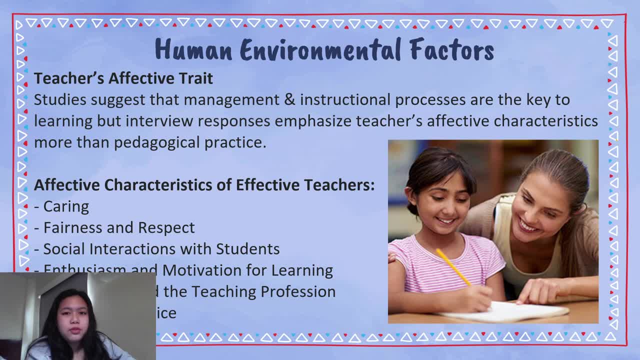 teacher is the attitude toward teaching profession. are you dedicated to that kind of profession? because if you're not, then it will surely affect your students performance, your students motivations. next, reflective practice. so you, as an effective teacher, you always have to reflect. tama ba yung ginagawa ko. 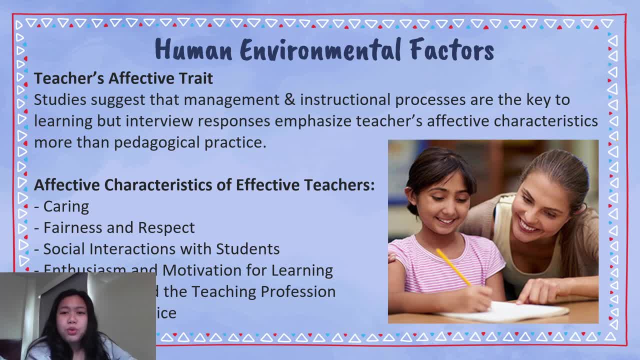 tama ba yung pag tuturo ko. yes, you always have to reflect. now imagine if your teacher is not caring, not fair, snobber, boring or not dedicated with his or her profession. that will surely affect child's or the student's motivation again and again. human, environmental factors. 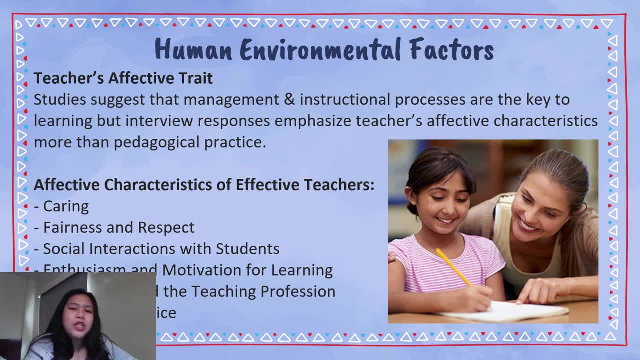 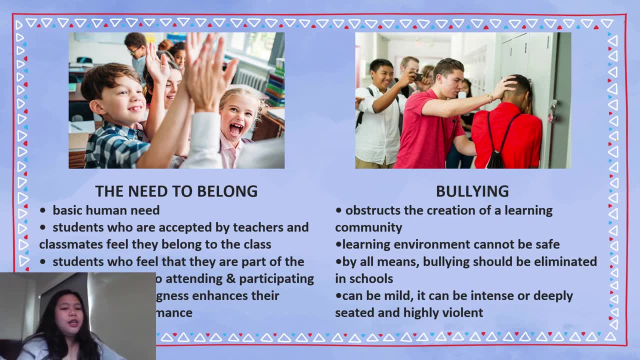 has always this effect towards the student, especially you as a teacher. now let's move on with that. let's continue with this. the need to belong. everybody read the need to belong. now. this kind of feeling is a basic human need. for example, ako i'm a christian, right, i'm from. 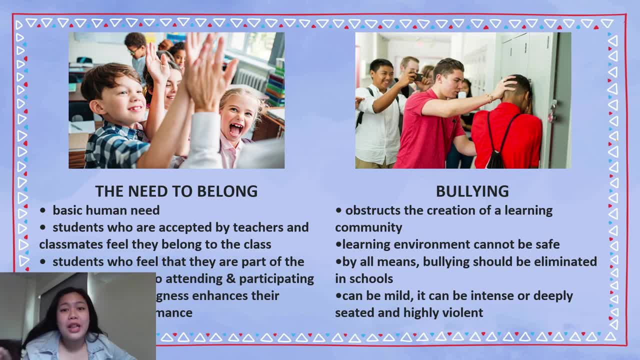 pagadian city and i manage myself to enter msu, mindanao state university of marawi city, which is an islamic, islamic um area. now i always have this feeling the need to belong, because so far i'm always out of place. out of place. 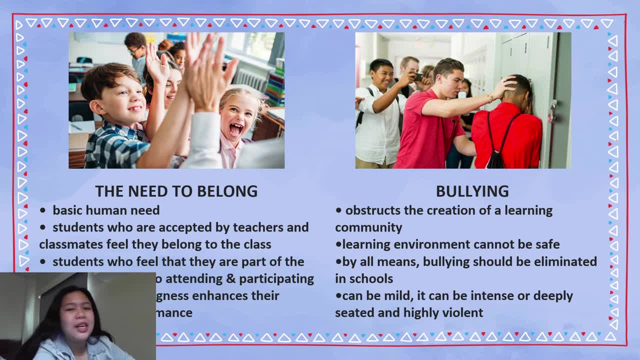 number one: the language. i can not speak with their language, so i am not belong with them, right? number two: they are muslims. i cannot relate to them. we have different beliefs, so in my mind i usually before, before, when i was new in msu, i always had this: 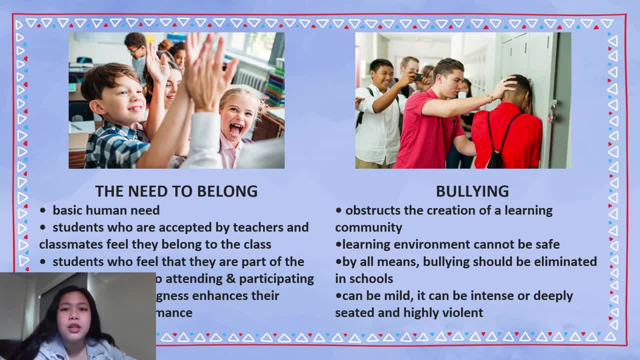 mind to find christians so they can understand me. like that you get the point. i always have the urge during that time. i always had the urge to be belong with a group that can understand me, that can relate with me, because, again, that is basic human need. 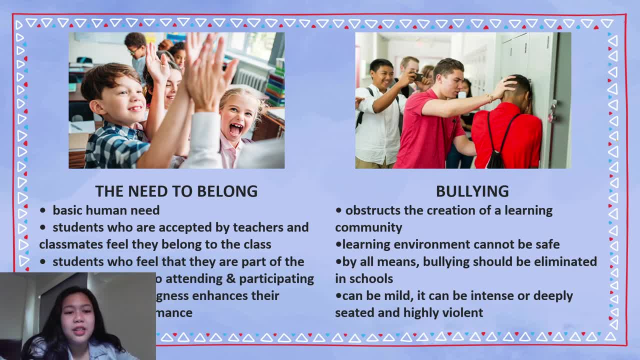 same as with our young learners, they need to feel belong because if they are out of place it will really affect their motivation again. students who are accepted by teachers and classmates feel they belong to the class. students who feel that they are part of the class look forward attending the participating 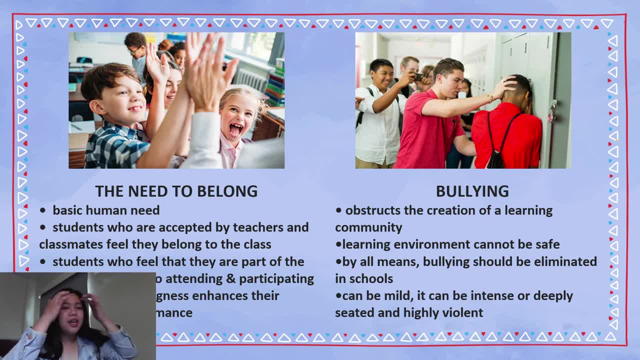 no example. usually what happens in traditional classroom: the teacher is the only one who answers. the teacher is the only one. it's like teachers just focusing modeling, molding. those students who are already capable of molding themselves by themselves and those who are not- low achievers, are left behind. 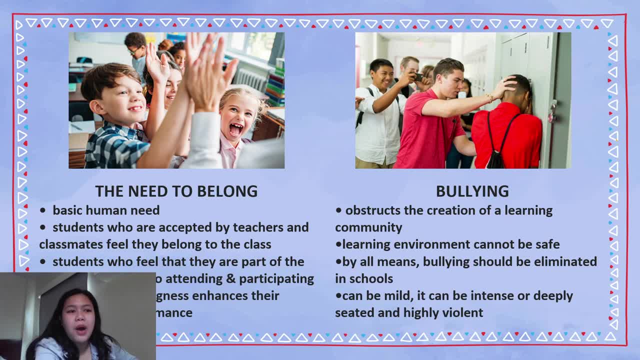 because they are not. they are the ones who give. so, as a teacher, inclusivity- everyone should be included. no one should be left behind. again, sense of belongingness enhances their learning and performance, not because they are weak. don't include them. they can't answer no, you always have to feel. 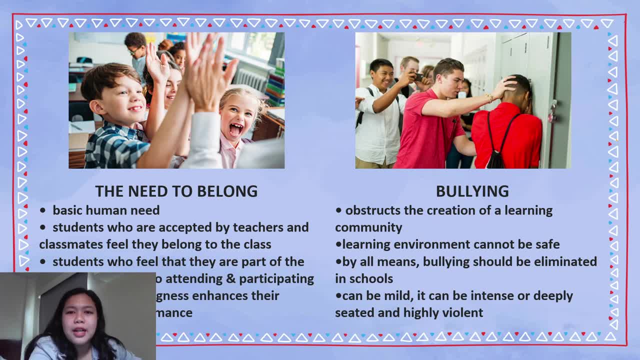 make them feel they are, belong with us, they belong to this class. they are, they have this capability and, as a teacher, it's your job to bring that out. so, yes, another another human, environmental factors are bullying, of course, especially elementary students. I am a victim of bullying. 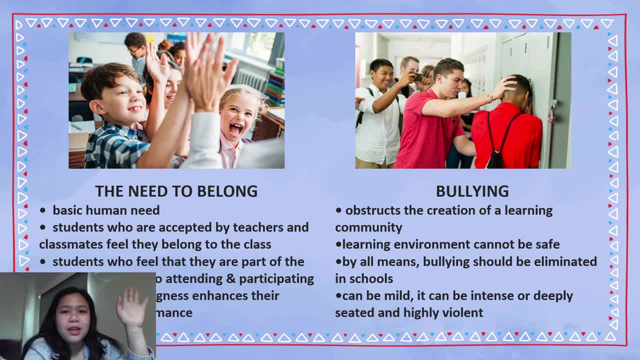 who else? um, in my case, I'm always bullied because of my physical appearance. I am very chubby, I'm fat, yes, I have this big body and a flat nose, which makes me look like a pig- and at first I wasn't. I wasn't really. I really can't handle that bullying. 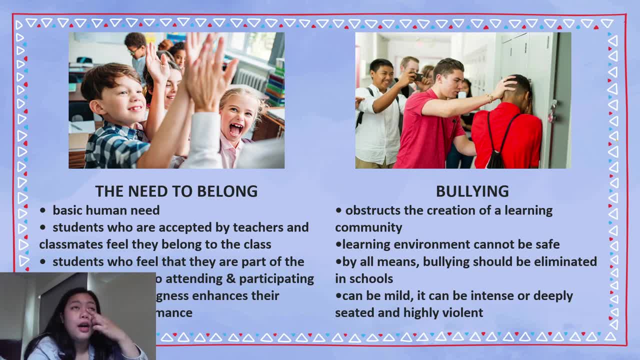 when they say baboy, baboy, baboy, baboy, I begin to self-pity myself, self-pity myself. that happens and I don't want to hear it. I make excuses, you know when, especially when I get near to a group of students always bullying me. 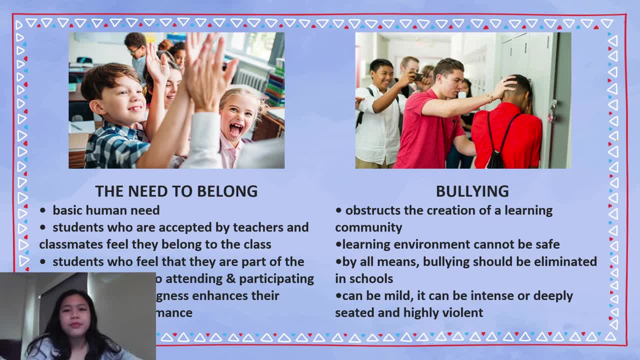 I'll be like twing, get out of their way. when I see there in the classroom, I'll be like I'm not feeling good with this one. okay, especially when I feel like I'm going to be bullied again. I'll leave the room. turns out cutting class. 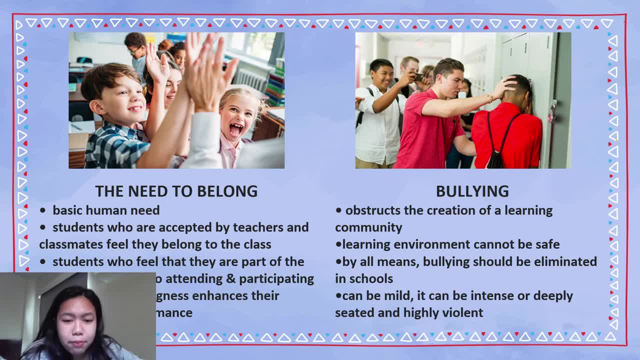 so I have. I don't have the motivation to go to school because there are people who are always picking me up: baboy, baboy, pig, lawas, yes, ugly. so again, bullying obstructs the creation of a learning community. they feel again like they don't feel. 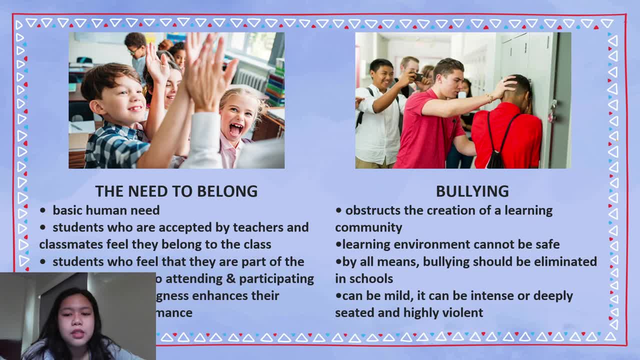 belong. they're always the outclass. the learning environment cannot be safe. it is not safe for them. why it affects here. it affects their mentality. take it from me as a bully victim for years, from from grade 1 to grade 12 and even until now as a college. 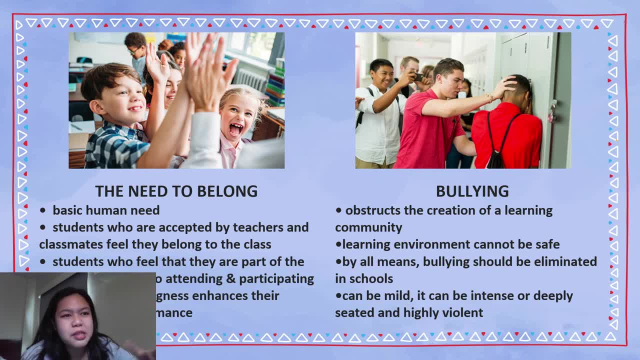 third year college. I somehow get that. but college I don't really mind, because I am somehow improving my self-confidence, also with the help of people, lovely people, who build my confidence. and yes again, by all means, bullying should be eliminated in schools. as a teacher, always, always. 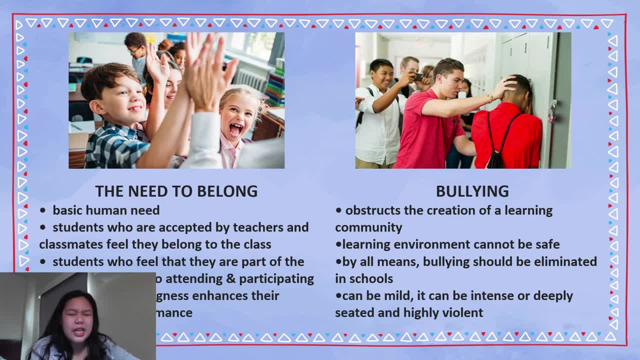 do not tolerate bullies. okay, if I hear the bullies don't do it. it hurts the bully. they also need care, proper care, properly you should have. you should handle them well, because if you push them you will hit them. oh, that's bad, you're very bad. 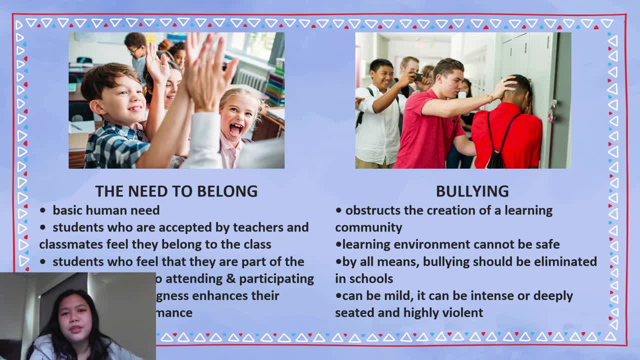 you're a piece of like that. don't be like that because it will be triggered. maybe it will get worse. so handle the bully victim and handle the bullies. there are seminars how to handle bullies, especially young students. they don't know yet they are like that. 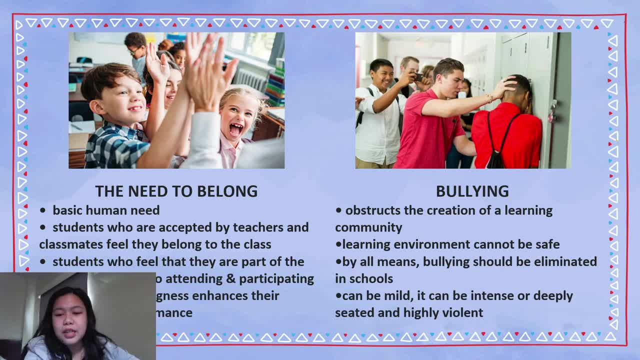 so yes, again, bullying can be mild, like bully. bully hit him, hit him in the head, hit him like that, but the feeling of victim bullying is like he's getting hurt, or it could be intense or deeply stated, highly violent. so that's where it goes, the modification. 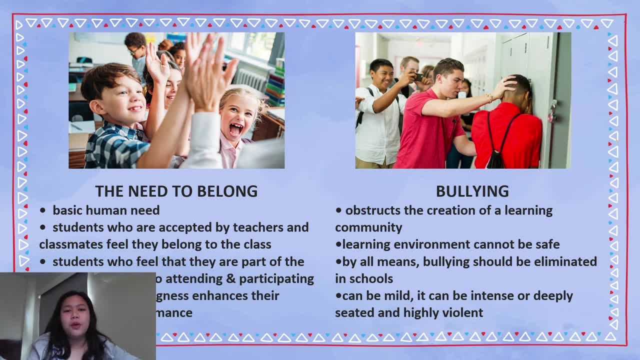 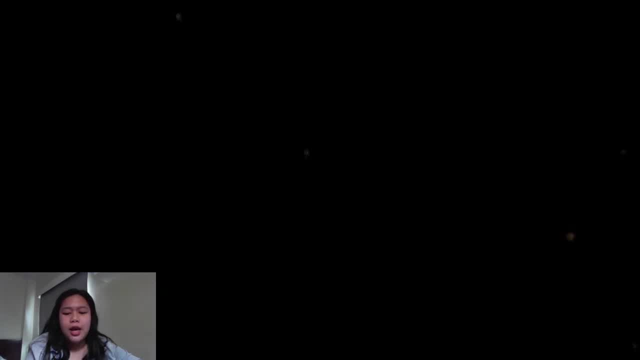 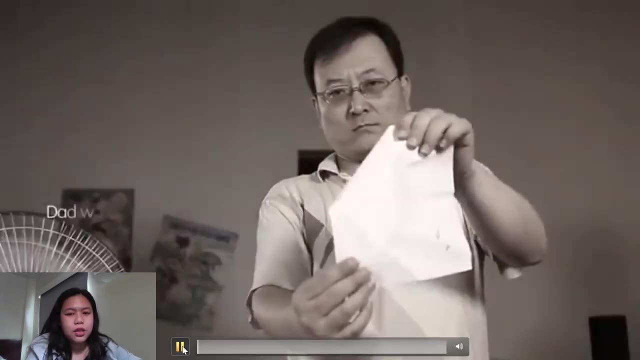 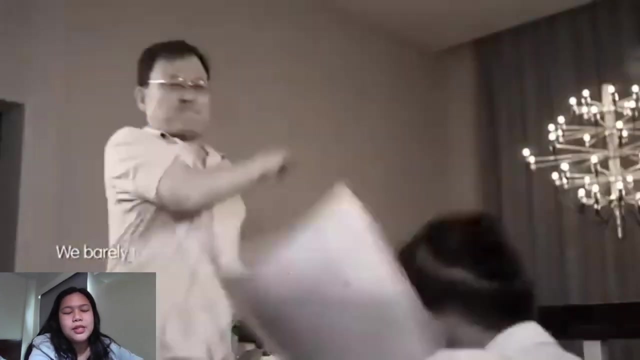 I mean punching, individualize, humiliate, humiliate anyway. so, Um, we still have another part. I have here a video that you should watch and tell me what you think. What's the? what's the? tell me what's the message of this video. 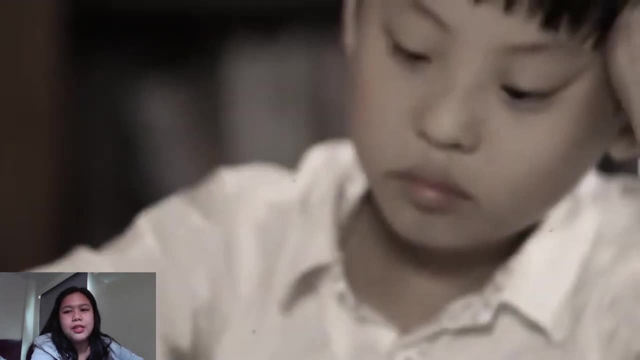 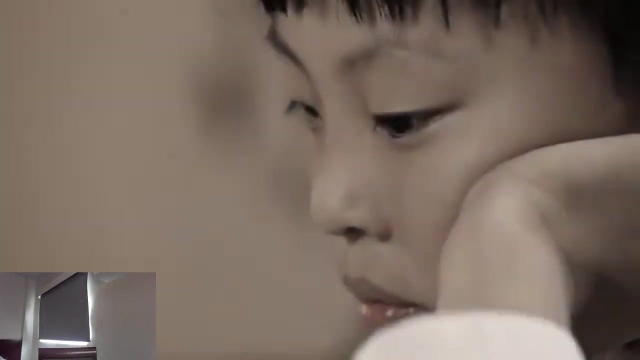 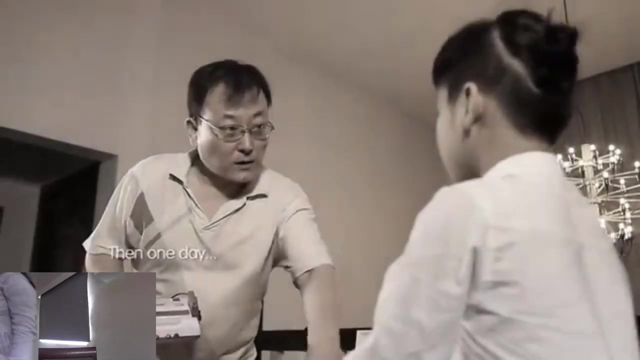 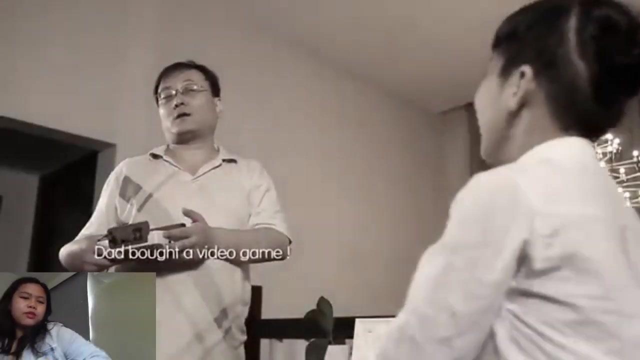 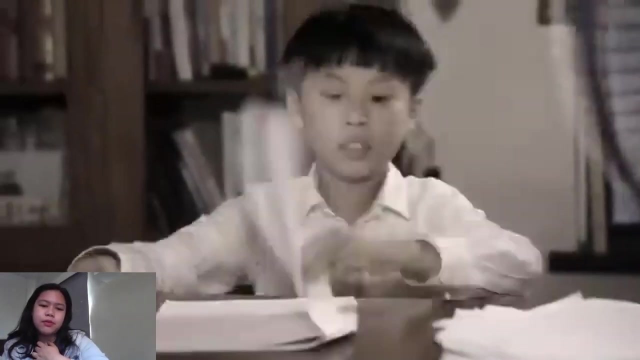 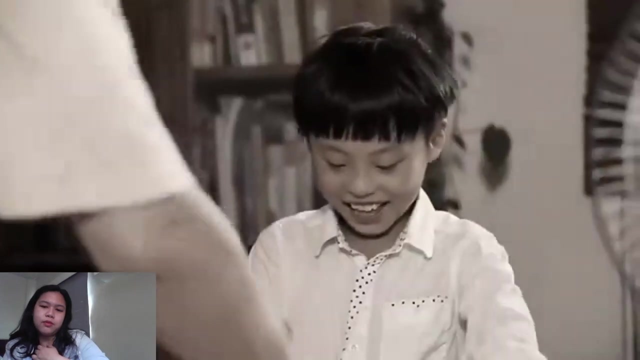 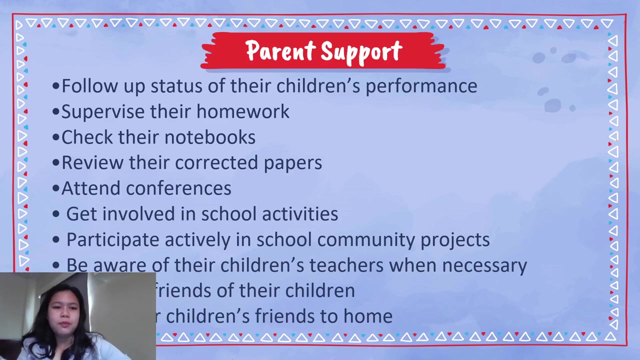 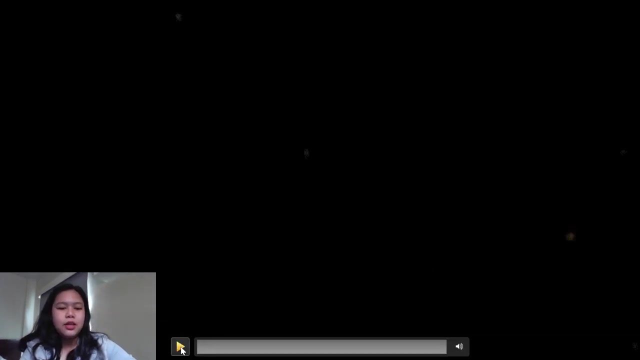 As you can see, there's a father who ruined his output. Wait a minute, Wait a minute, Wait a minute. So, yes, you can see the PPT, Anyway. so at first you can see that his father is not supportive of his output because he's not doing his job. 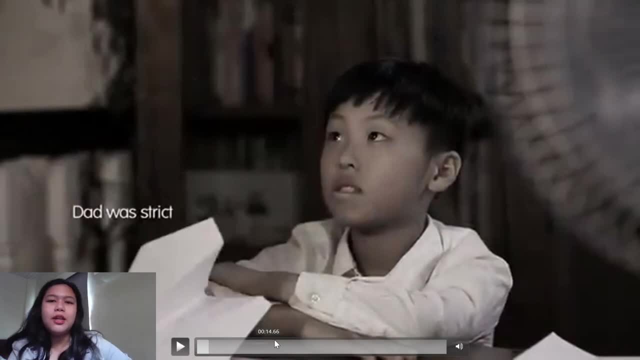 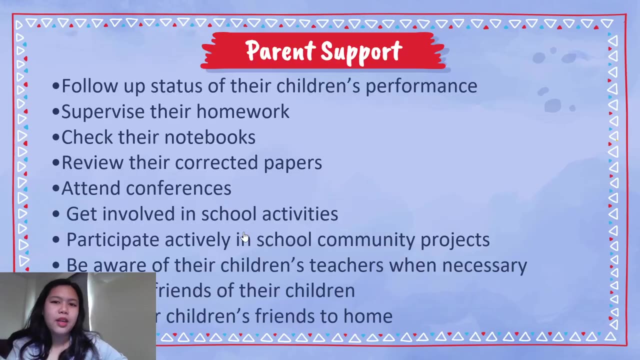 But right after that, the father did something like a reward. If he does this, he will give this PlayStation to his son. So the point here is: parents are always involved In learning with our students. Now we call this parent support. 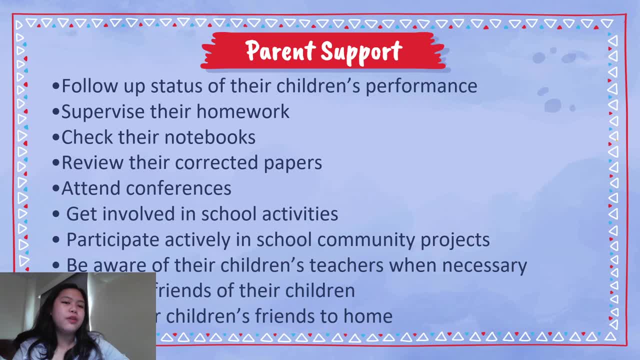 Now, what is parent support Number one? it should. how do parents support Number one follow up status of their children's performance So it could be talking with their teacher? Ma'am kumusta, yung anak ko, Ganun choo, choo, choo choo. 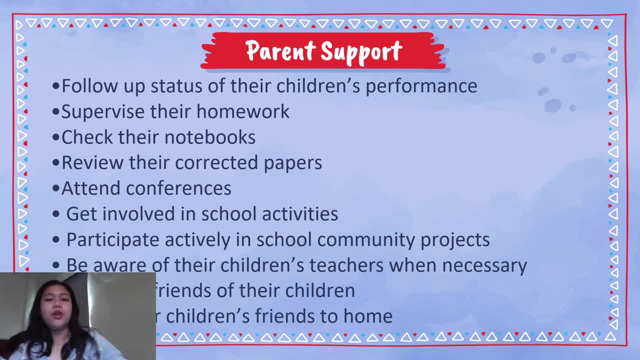 Next, it could be supervising their homework. Pag may homework yung anak nila, they can help them. could help them more, Just guide them with their assignments. Number three: check their notebooks. So yan, Have you tried a notebook before na merong nakalagay dun sa baba na parent signature: choo, choo, choo. 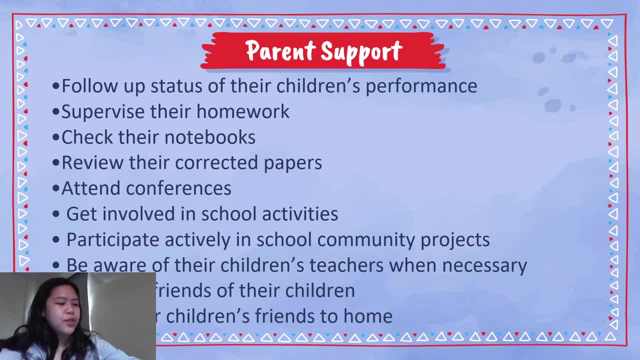 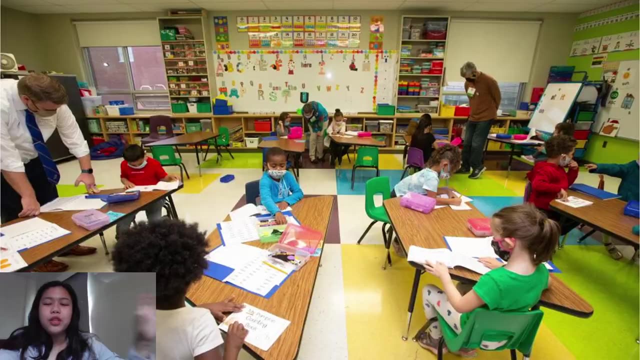 So yes, most commonly it happens in lower grades or elementary grades. So chinecheck din yung notebook nila, Able to know if their students are jotting down notes in their during the discussion of their teacher. Next review their corrected papers. 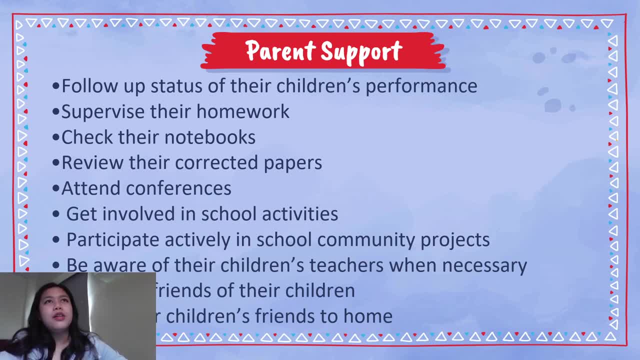 So when we say corrected papers, it could be the sit works like quizzes or test papers, ganun. So doon din ang mamonitor ng mga parents, ang mga anak nila. Next is attend conference. So Ito yung meeting. 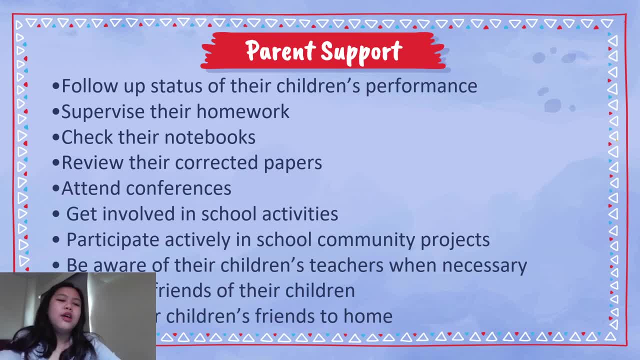 Ganun Parent Teacher's Association, So doon na bibigay ng na-ask the mga parents yung mga concern nila about their about their children, And then yung teacher din mag-re-report kung anong performance ng kanilang anak sa klase. 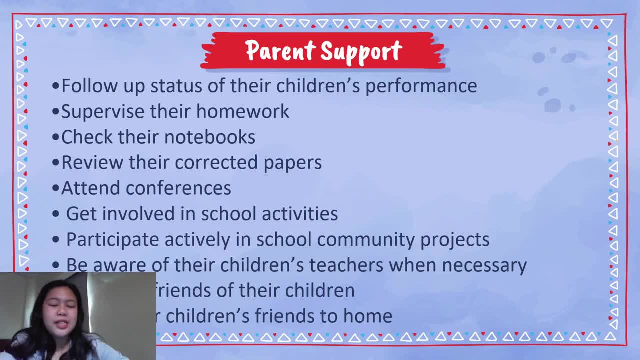 Next, get involved in school activities. So example: nyan is family activity. So, ayun, I've never experienced that, I've never experienced that before, But yes, there is family activities in school. Next, participate actively in school community projects. 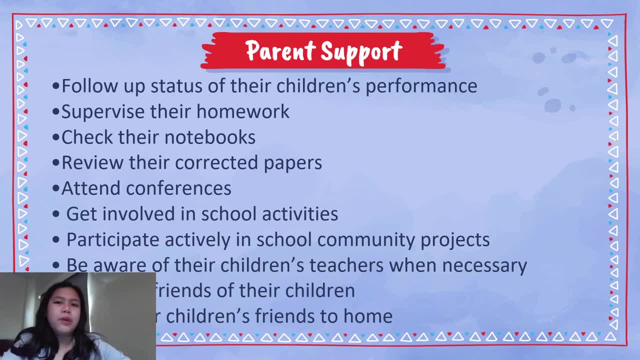 So iba din ito Community projects. It could be tree planting, whatever. Next, be aware of their children's teachers when necessary. So again, be aware of their children's teachers. So example nito: Pag magsumbong yung anak nila. 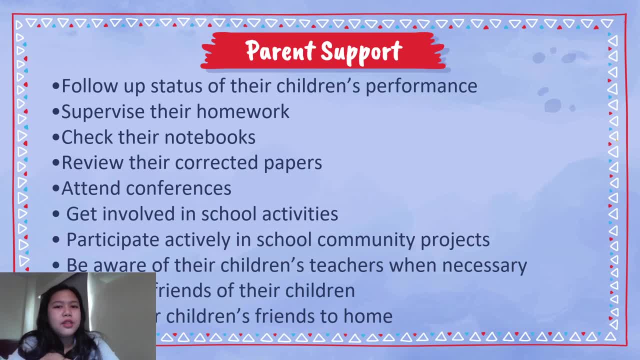 Anak nila na ma ganito si teacher ganito ganyan. You should always be aware of that. You could always confront the teacher na Ma'am, ano tong sinasabi ng anak ko na ganin-ganin. 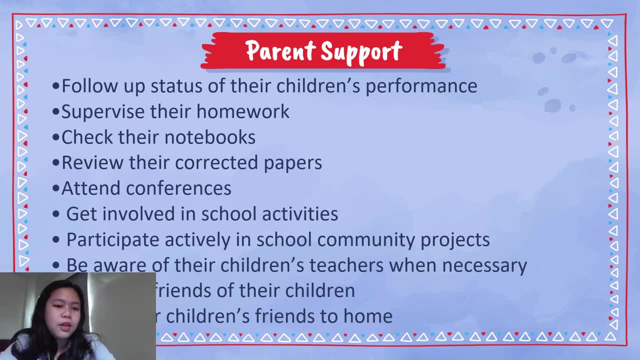 So that's an example of parent support. Next, meet the friends of their children. Okay, ito, Meet the friends of their children. You know, as in hindi pa naman ako parent, Pero most commonly nakikita natin sa mga parents. 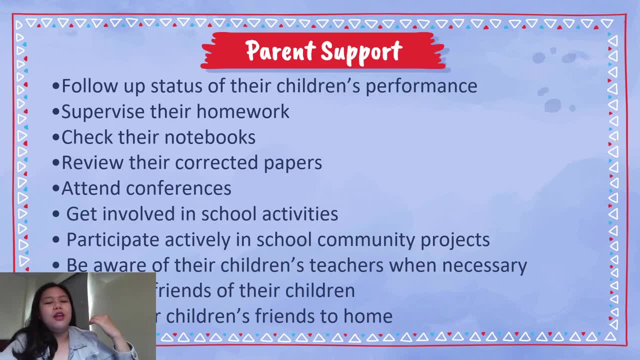 Most commonly nakikita natin sa mga parents natin na They're very keen, what you call this. They're very um napipipili ba kung anong circle of friends Where their children belong with Na kung mabuti ba or mabasagulero ba. 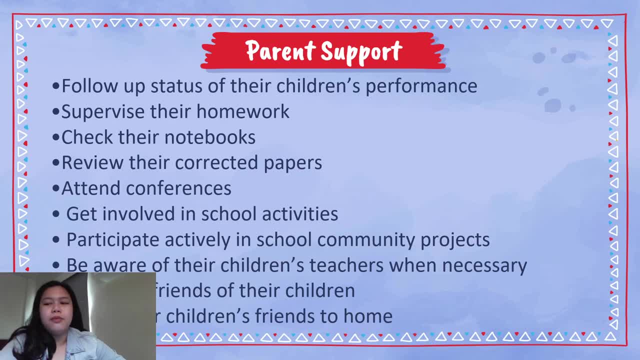 They are very ano um nakikikulado sa tao nyan. And yes, But as a parent, you should always um be open-minded of their group of friends or circle of friends, And next you could always invite their children's friends to home. 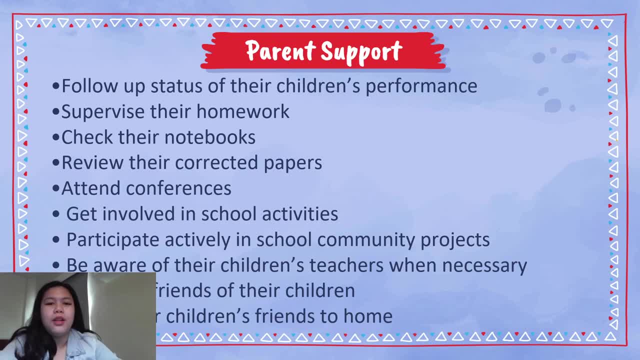 So wag mo masyadong pagbabawal, Kasi kung hindi mo, um if you wouldn't try this one, Most commonly yung nangyayari: yung mga anak nila mismo magpupunta doon. 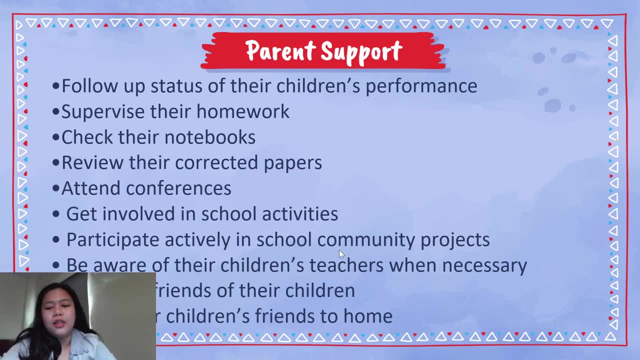 Laan doon. So, yeah, try that And maybe it could improve your um students- I mean your children's performance in school Now showing your support as a parent. So madami ko ang dami ko nang sinabi sa parent support. 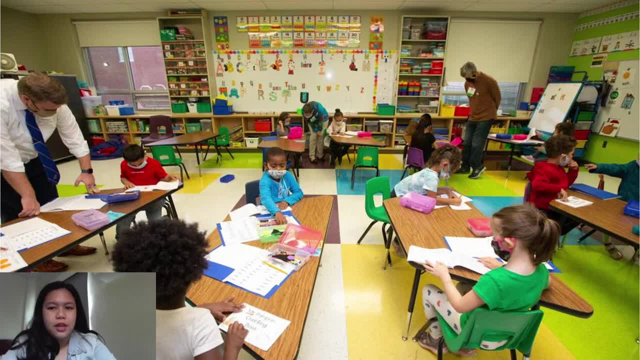 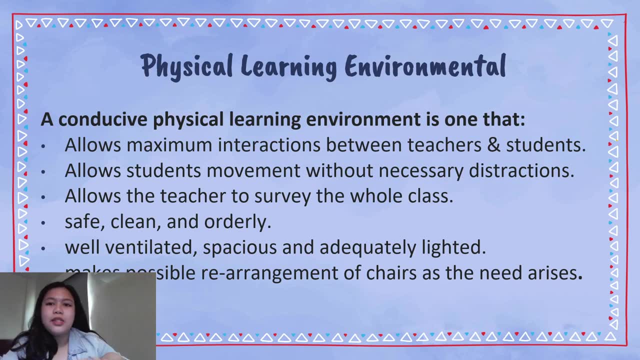 Let's move on to what is this? Okay, the physical learning environment. So I can use the physical learning environment. By the way, this is the last one, no, Uh, environmental environment. So what are the environmental factors that could affect the motivation of our students? 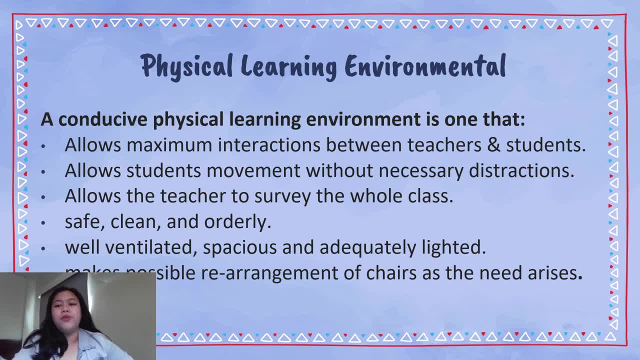 Number one allows maximum interactions between teachers and students. So the environment, or the classroom mismo, should um allows maximum interaction between teachers and students. Next, allows students movement without necessary destruction. So this, this is where um 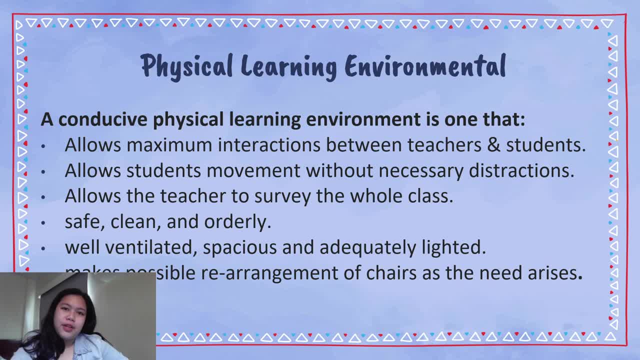 the arrangement of our furnitures, or the, the chairs, the tables of our students. Mga lalagyan natin, It should be. there should be, um, what do you call this? There should be, um, uh, a space that they can move around freely. 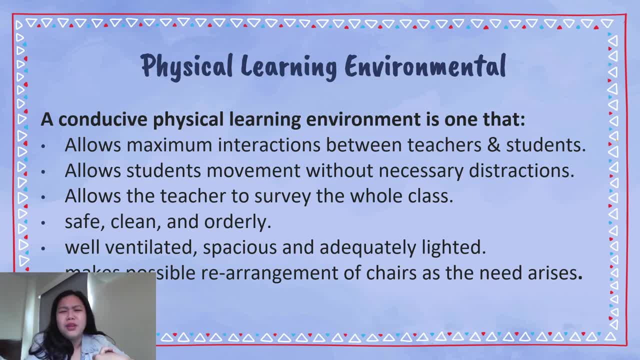 Hindi yung masyadong. ano mo taw nito. Masyadong maliit yung daan, Maliit yung daan So they cannot move. And next allows the teachers to survey the whole class. 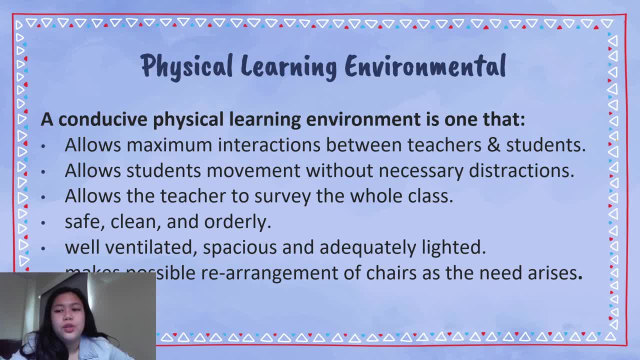 So yes, you, uh, the teachers should always survey the whole class Next, safe, clean and orderly. Now, when we say safe, hindi lang sinasabi natin yung pag may mga masaker Diba Uso yun sana eh. 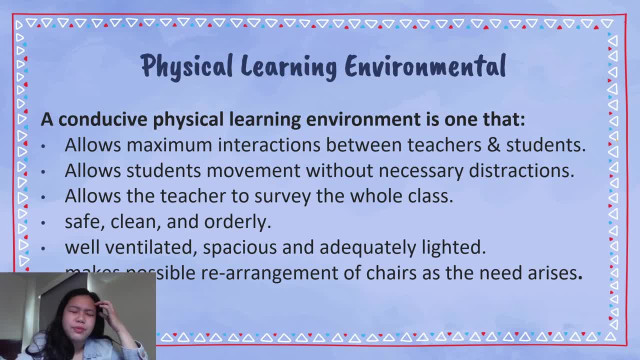 Sa sa Amerika meron tinataw na like. I think this happened last year lang. May may pumasok sa classroom rin na pinagbabaril yung mga estudyante, Anong tawag nito: Gun Shoot, Shoot, Parang ganon. 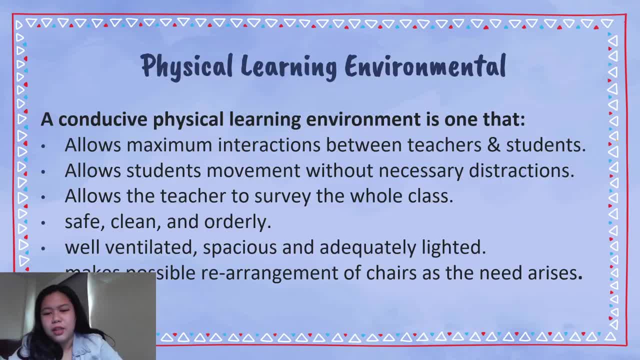 Um, yes, it's not just about that. Um, I mean, I'm not just disregarding that kind of safety, no, But dito sa Pilipinas, wala namang ganon, Wala namang ganon. 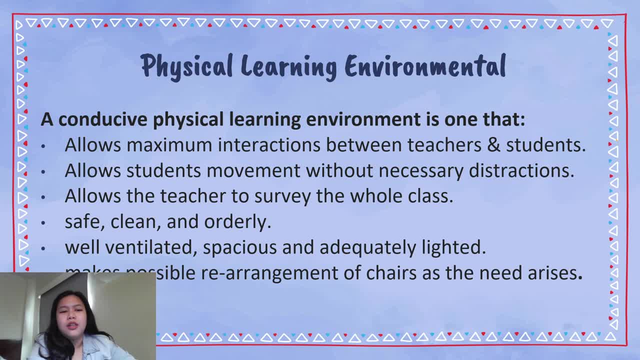 Wala namang gago na humapatay ng mga estudyante. Uh, thank God, But um. another. another term of the safety is example: putting sharp, sharp things in your classroom. Now you shouldn't um as especially sa mga young, young or mga lower grades. 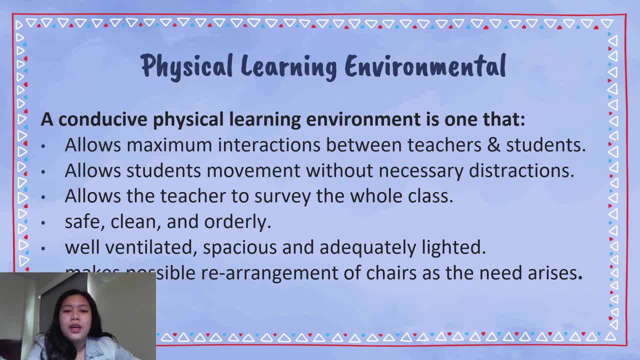 you shouldn't. you should be careful with that thing, Because what if, for example, may glass ka dyan na basta tapos? they will run over it? It's not really safe for them to be uh around with it. 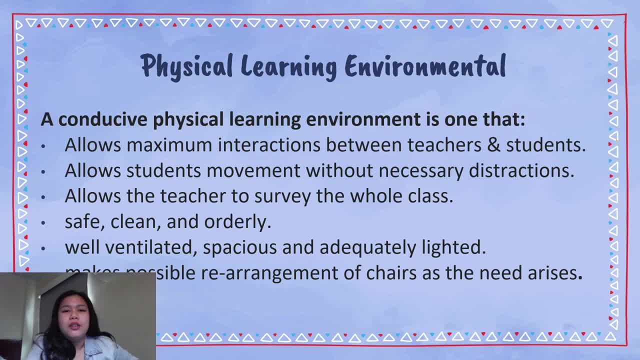 Next, clean. Okay, The CR should always be clean. Number one, yan, The CR should always be clean. The floor, their tables, their- uh, their chairs. no, Because that is to avoid disease. And next, orderly. 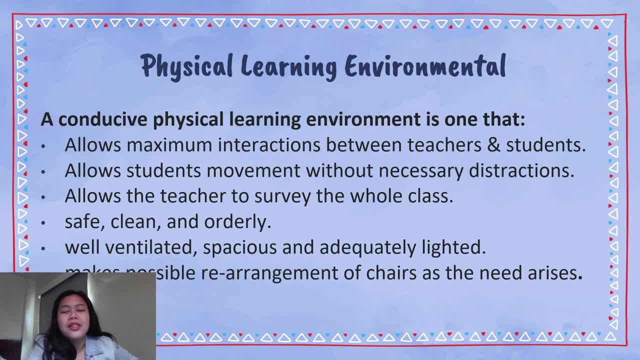 Again, the arrangement, The arrangement of everything inside the classroom is very, very important. Kasi, that will um when. when we are order with our things, when there is proper order with our things, then it will avoid any accidents. no, 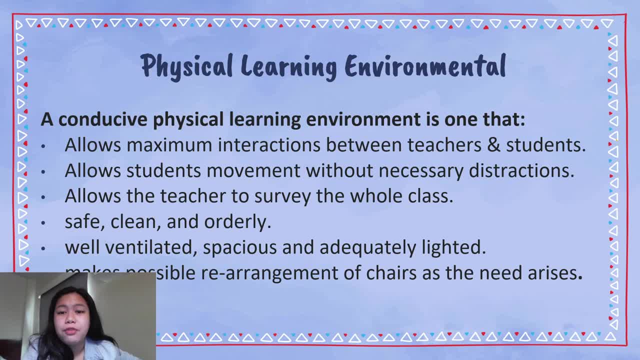 Or any uncomfortable environment feeling. So yes, Next let's move on to well-ventilated, spacious and adequately lighted Okay. Ito ang number one concern ko Kasi when I was uh elementary. I swear to God, parang hindi ako makahinga. 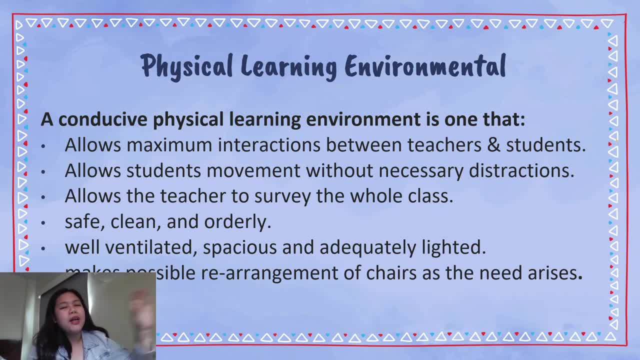 Bakit Yung window like parang window siya, but it's just grills, It's just steels. But ang ginawa ni teacher before is tinakpan niya ng kung ano-ano Like dinasplay niya yun, yung mga illustration board dun. 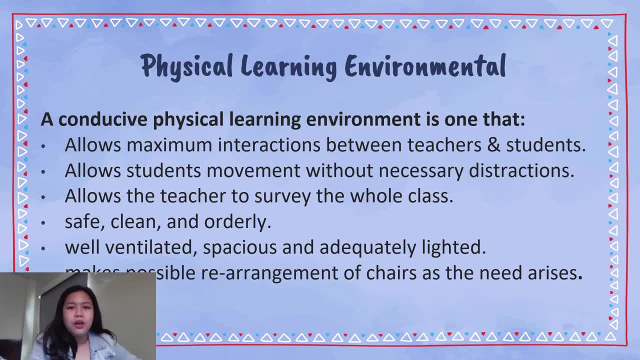 And it turns out walang proper ventilation of air Diba. So ang nangyari: napaka-init ng classroom, napaka-baho ng classroom, especially pag, um, especially pag lunchtime, Tapos yung mga boys namin ang ang amoy araw. 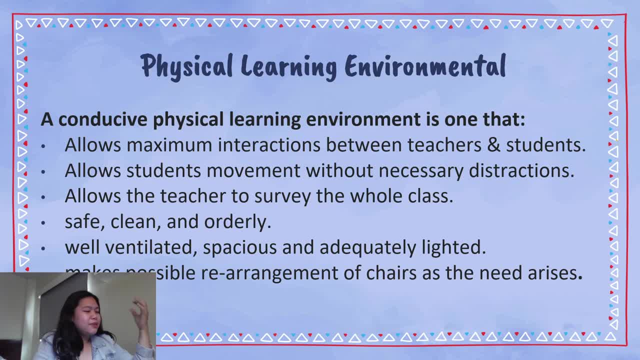 amoy, anong tawag ito? Um basta amoy, araw maewan ba Tapos walang proper ventilation. Diyos ko, doon Tapos yung mga window, pa namin giba-giba pa. 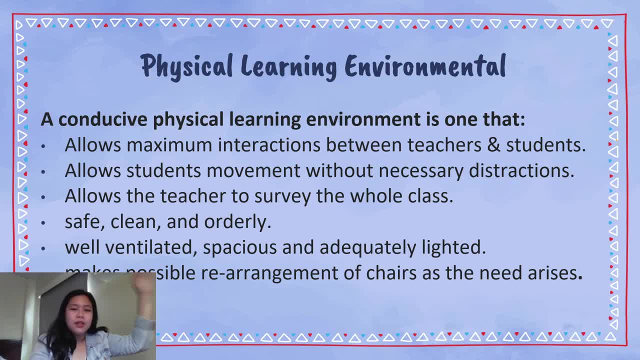 Yung iba nasisirado hindi nao-open Ganon. So again, teachers, ventilated classroom is very important, no Kasi, para there is fresh air. Pag fresh air, fresh din yung utak ng sudyante. 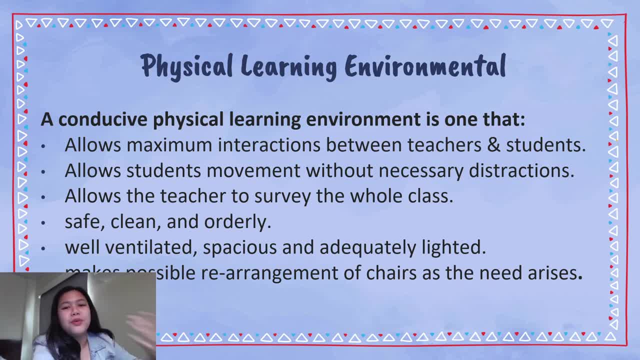 Ganon lang yun Next spacious. So paulit-ulit natin sinasabi: Do not put unnecessary things, Put unnecessary, unnecessary furniture inside your classroom. I will tell you: do not put refrigerator inside your classroom. It's not, it's not necessary. 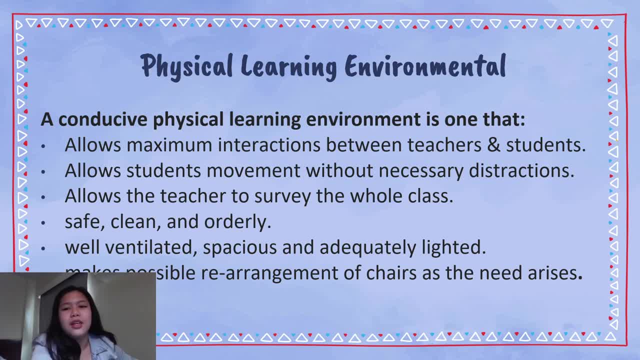 Do not put tables in your classroom. It's not necessary. Uh, the more spacious, the more, the more. anong tawag ito? Much better, Much better, kasi nakakapag ano yun, nakakapag move yung whole class. 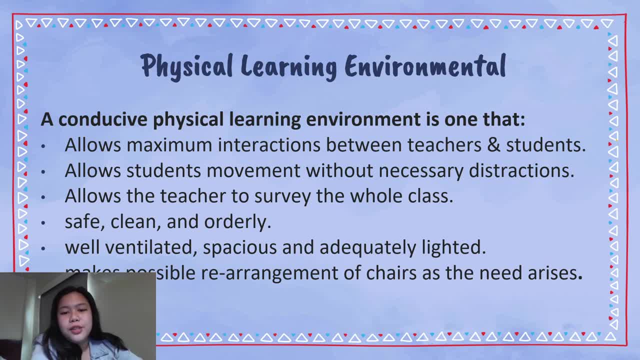 Next adequately lighted. Okay, So tayo, mga public school, no Sanay na tayong ponder-ponder na yung mga mga ano natin, ponder na yung mga light bulbs natin. But again, physical learning environment. it is very important that there should be enough light for them to see what they write, see their surroundings and see what's on the board. 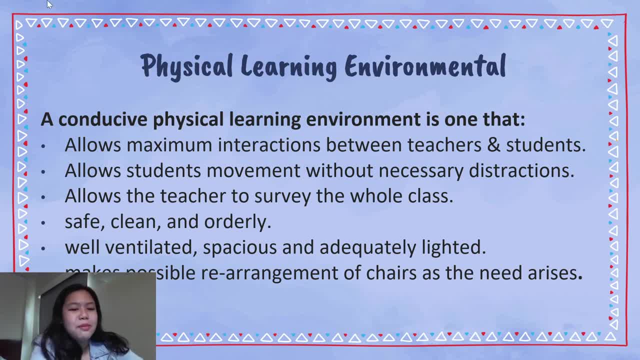 At saka makita yung kagandahan ni mga matyarat. Next, makes possible rearrangement of chairs. Arrangement of chairs as the need arises. So again, paulit-ulit na: Arrangement of chairs, So furniture, so on, so forth. 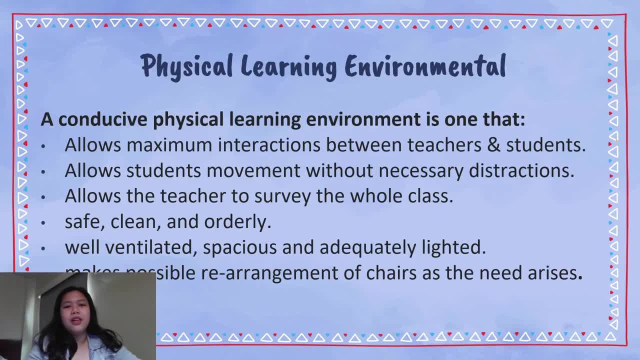 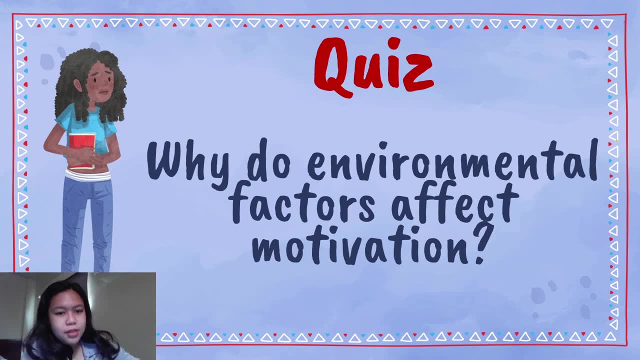 That is physical learning, environmental. Okay, Thank God, we're done. We have our quiz. This is very simple. This is equivalent to 10 points. Why do environmental factors affect motivation? So, based on our previous discussion- I think you have- you can answer this one. 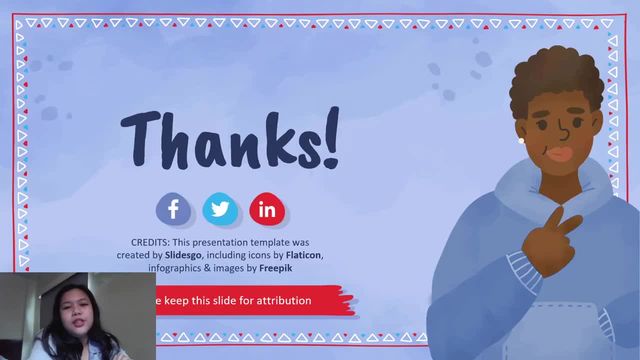 Why do environmental factors affect motivation? So that's it. This has been Nelmar Tumanda. Thank you for listening And don't forget to send your answers right away, because this is the last day of our what you call this basta mag, last of sa deadline na ngayon. 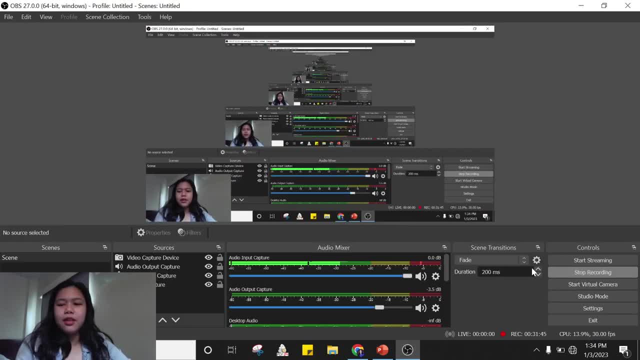 So thank you everyone, Bye-bye, Love you.